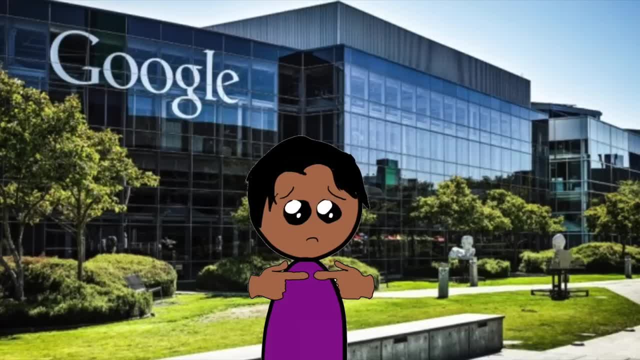 want to learn this. Don't do it to get a job at Google. Do it because learning this changes the way you think Data structures and algorithms, is about solving problems that you can't solve by yourself. So if you want to learn something new, you. 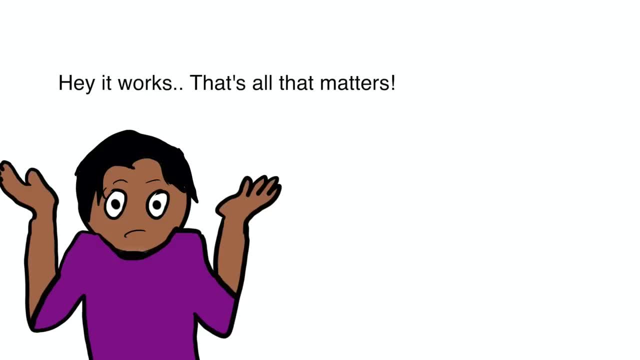 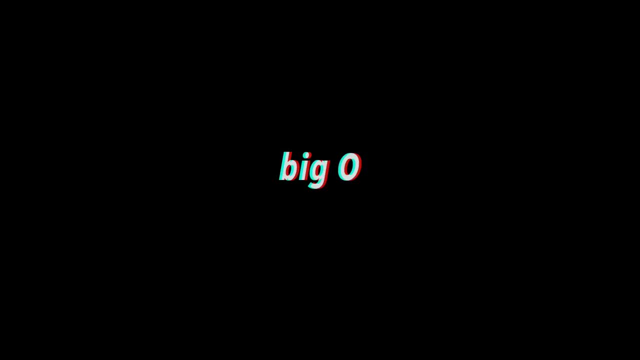 need to learn how to solve problems efficiently. A bad programmer solves a problem inefficiently, and a really bad programmer doesn't even know why their solution is inefficient. So let's start with that. How do we rank an algorithm's efficiency? Say we wrote a function that goes through every number in a list and adds it to a total. 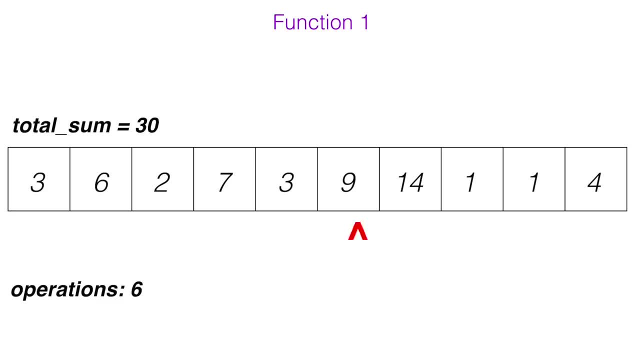 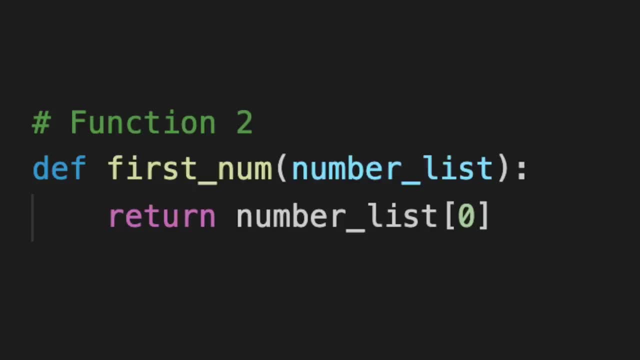 sum variable. If we consider adding to be one operation, then running this function on a list with 10 numbers costs 10 operations. Running it on a list with 20 numbers costs 20 operations. Say we wrote another function that just returns the first number in a list, Then no matter. 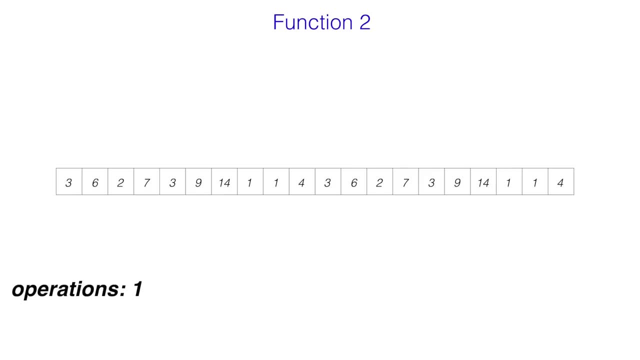 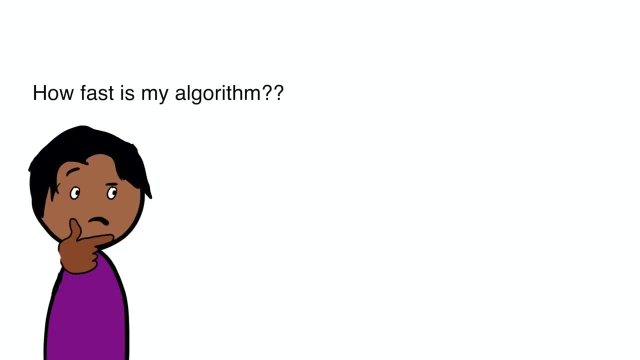 how large the list is, it's still a problem, So let's start with that. This function will never cost more than one operation. Clearly, these two algorithms have a different time complexity or relationship between growth of input size and growth of operations. We communicate these time complexities using big O notation, Referring to input size. 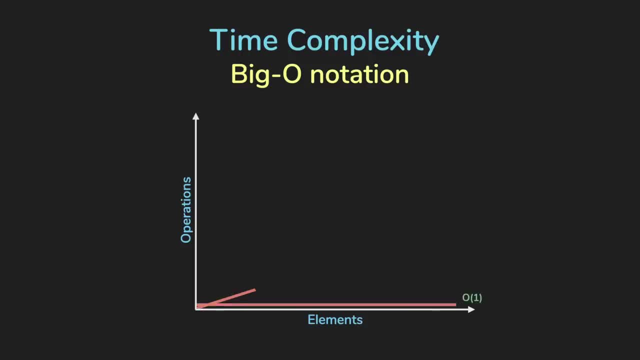 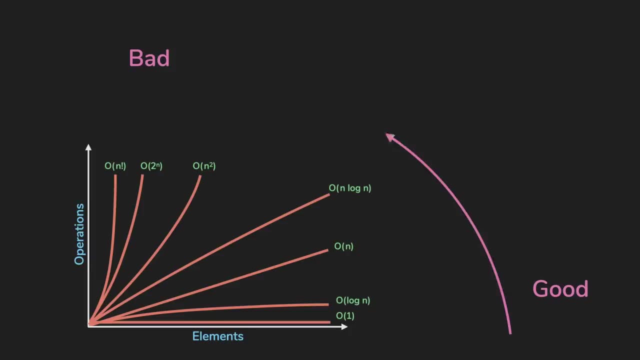 as n. common complexities are constant: linear, quadratic, logarithmic, n, log, n, exponential and factorial. Our first algorithm runs in O, meaning its operations grow in a linear relationship with the input size, which in this case is 0.. 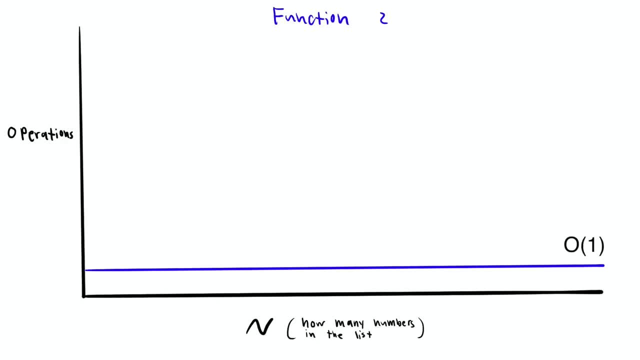 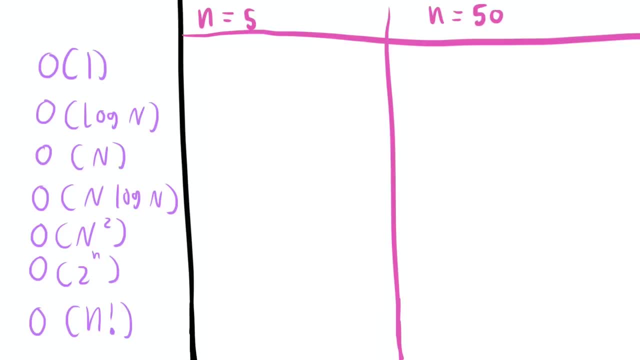 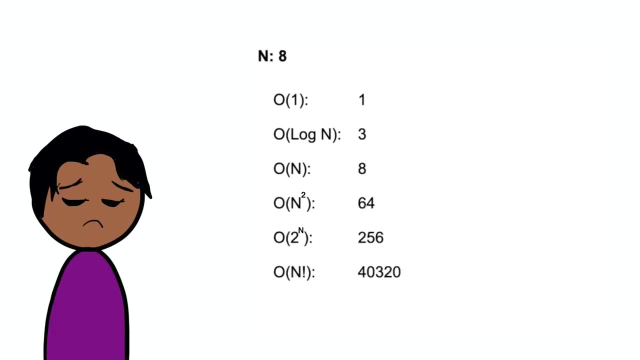 Our second algorithm is not dependent on the input size at all, so it runs in constant time. Let's take a look at how many operations a program will have to execute in a function with an input size of 5 vs 50. It might not matter when the input is small, but this gap gets very dramatic as the input 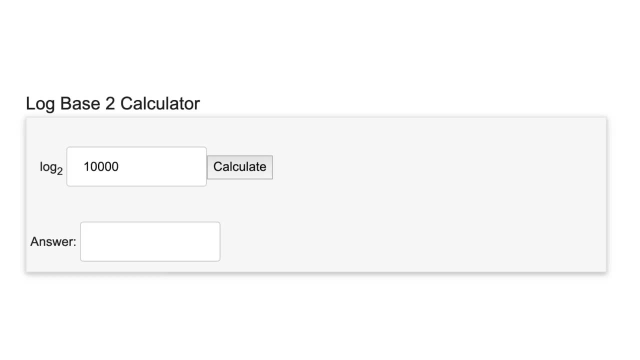 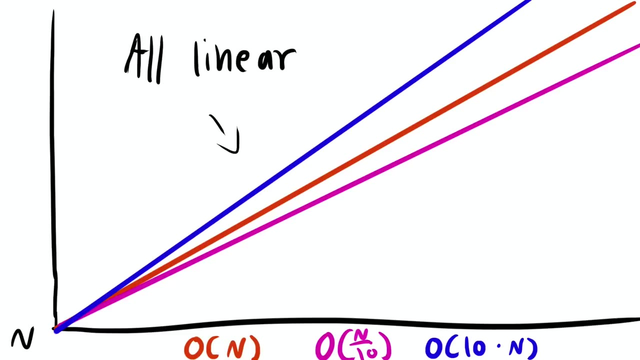 size increases. If n were 10,000, a function that runs in log of n would only take 14 operations, while a function that runs in n factorial would set your computer on fire. For big O notation we drop constants, so O and O are both equivalent to O because the 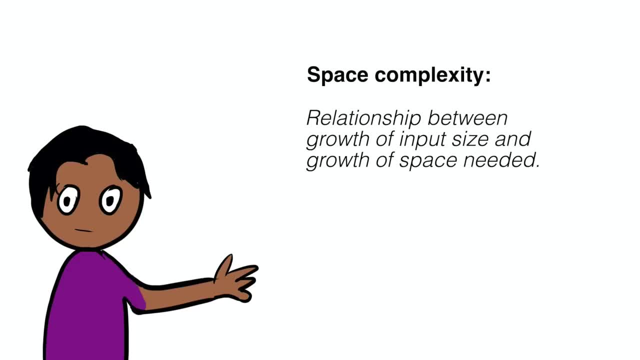 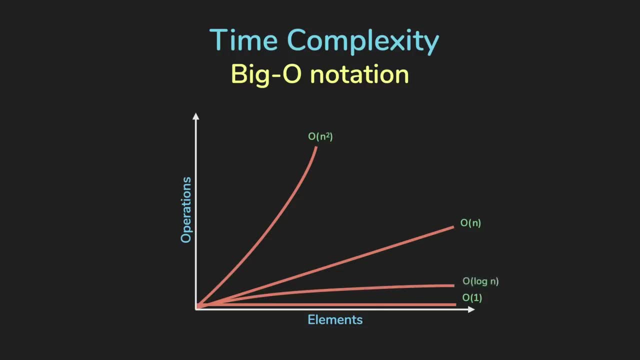 graph is still linear And big O notation is also used for space complexity, which works the same way for how much space an algorithm uses as n grows. Unless you sit in your room doing algorithms all day, there's a good chance you forgot what logarithms are. Logarithms are the inverse to exponential functions. Let's say I wanted 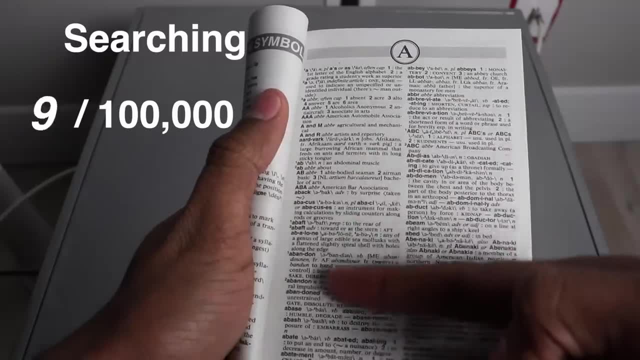 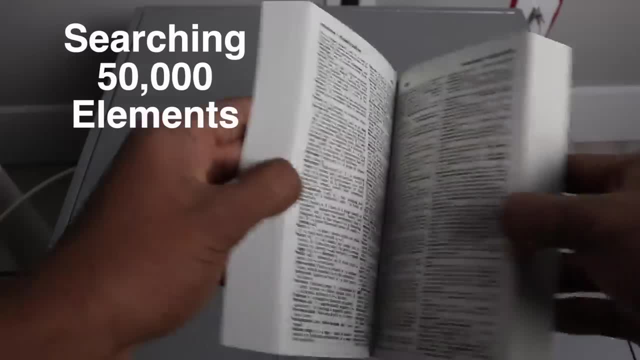 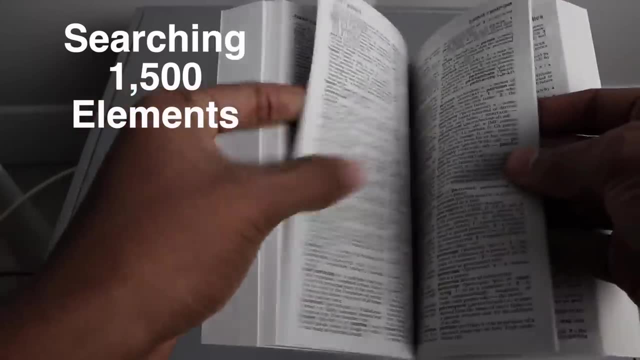 a dictionary with 100,000 words in seconds. We do something more along method 2. Cut the search window in half each time by checking the middle element. If we passed our word, search on the left half. Otherwise search on the right half, And then we repeat this. 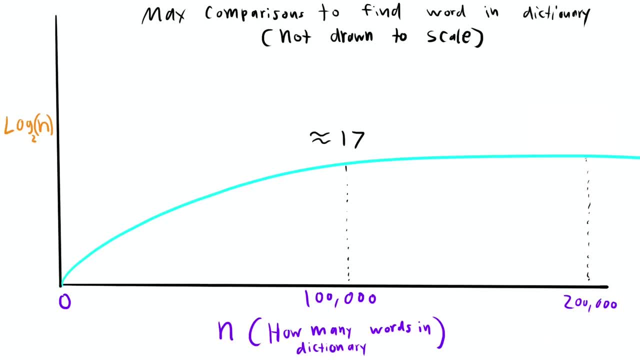 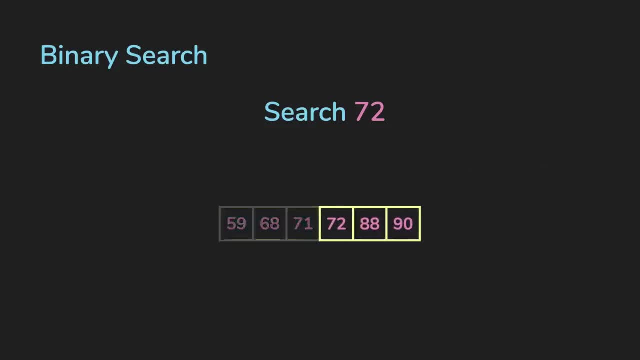 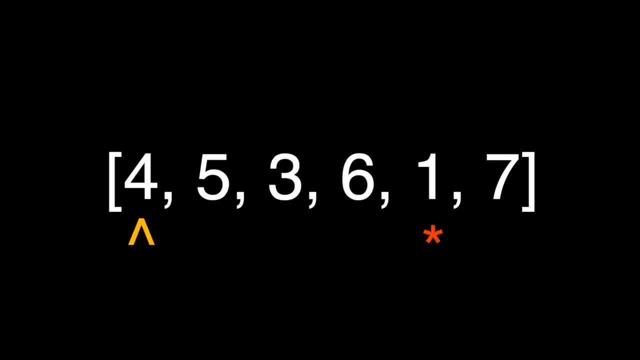 A very basic sort is the selection sort. You have one pointer at the start of the list and another pointer that is linear scanned to find the next minimum element. Then you swap those elements and increment the pointer, Since you're doing a linear scan for every. 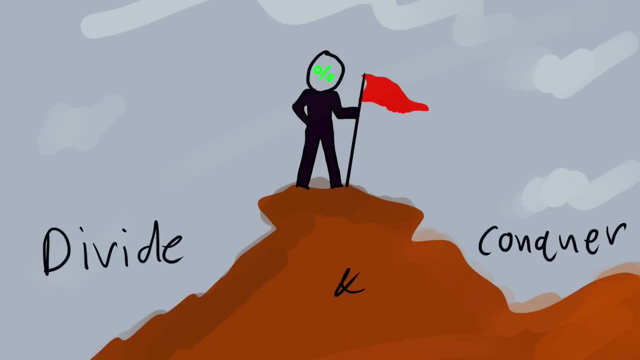 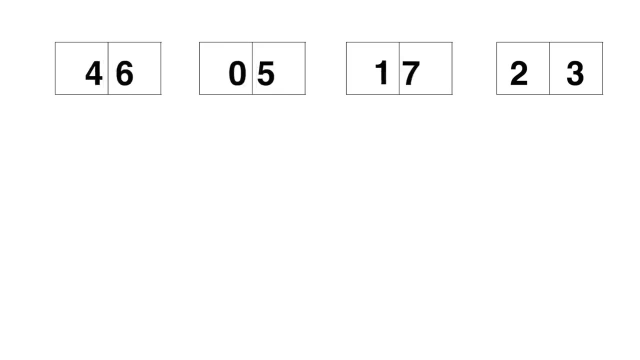 element in the collection. this runs in O. A more efficient algorithm is the merge sort. A merge sort splits a collection in half into sub-collections, until those sub-collections can be sorted in constant time, And then it works its way back up by merging sorted sub-collections. 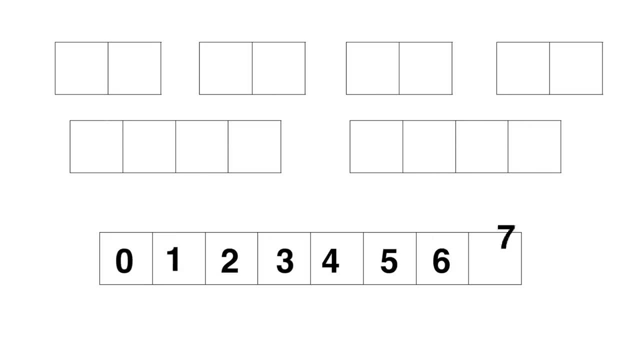 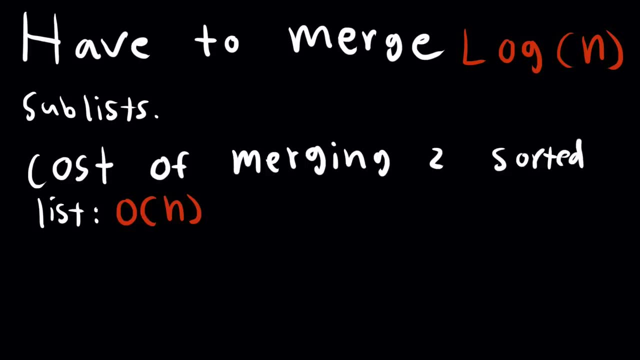 until the entire collection is sorted. Since it's splitting into half and half, it's in half, there will be log n splits and thereby log n merges. It is O of n to merge two sorted collections into one sorted collection. Since we're doing that log n times the time- complexity. 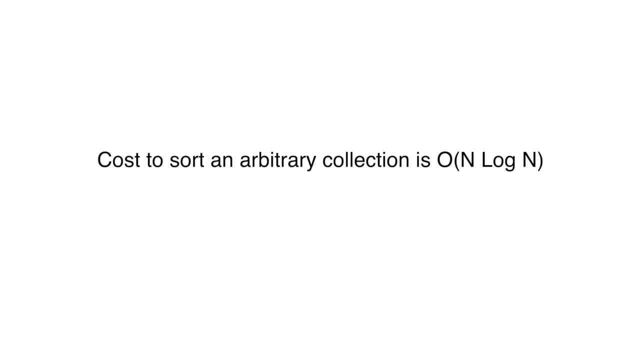 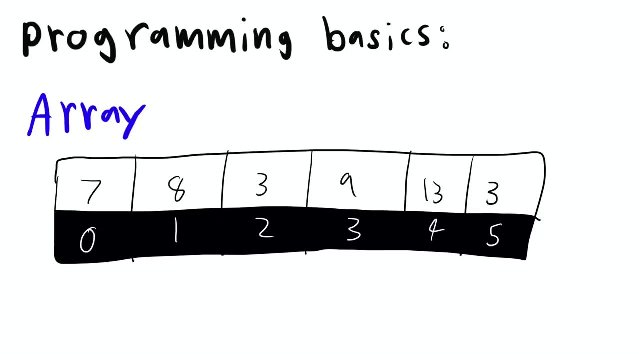 is O of n times log n. No algorithm can sort an arbitrary collection in a better time complexity than that, so we consider n log n to be the cost of sorting. Perhaps the most fundamental data structure is an array. An array is an indexable, contiguous chunk of memory. Arrays are fixed size. 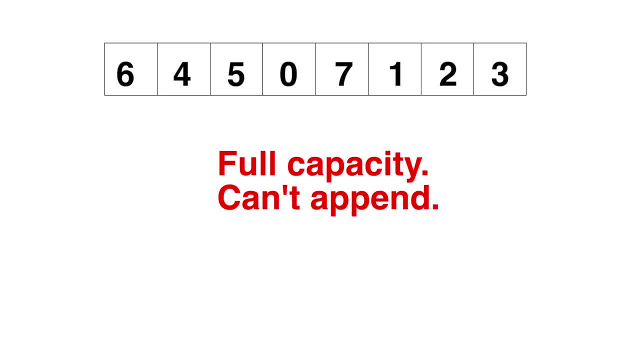 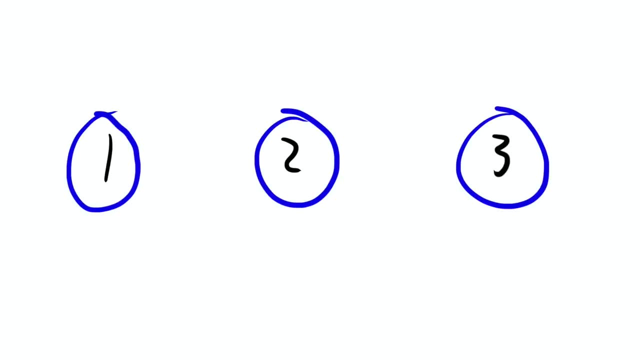 You can't insert a ninth element into an array meant for eight elements. A list data structure with a flexible size is a linked list. The idea is to package your data into nodes that hold one- your data- and two- a pointer that points to the next node Traversing a linked list. 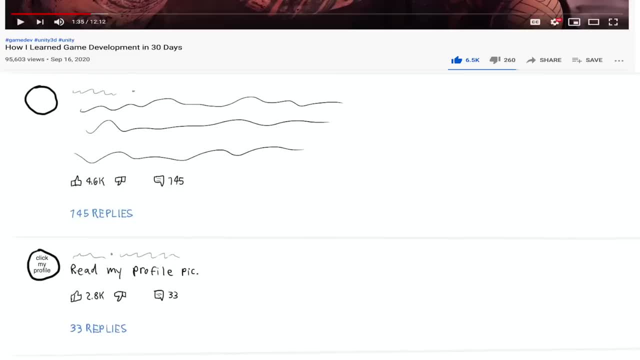 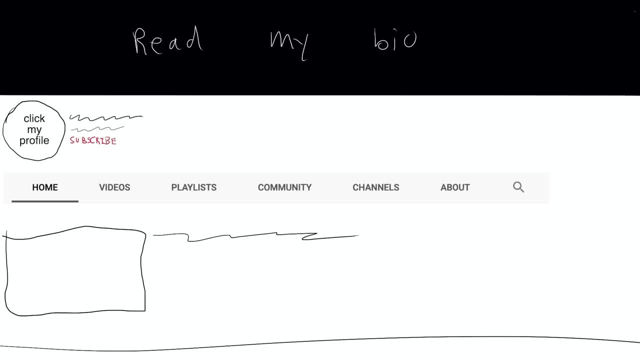 reminds me of those YouTube direction chains, Like you see a comment that says read my profile picture, and their profile picture says click on my profile, which brings you to their header, which says read my bio. So you go to their bio and it says: 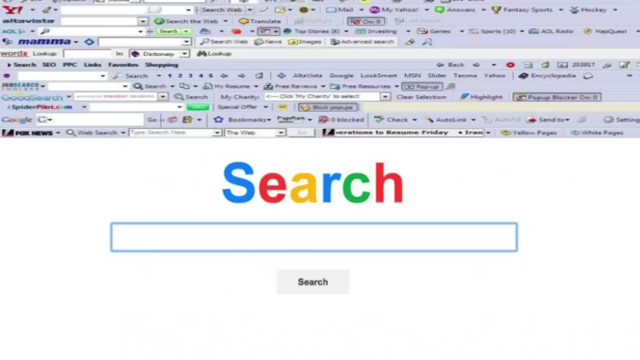 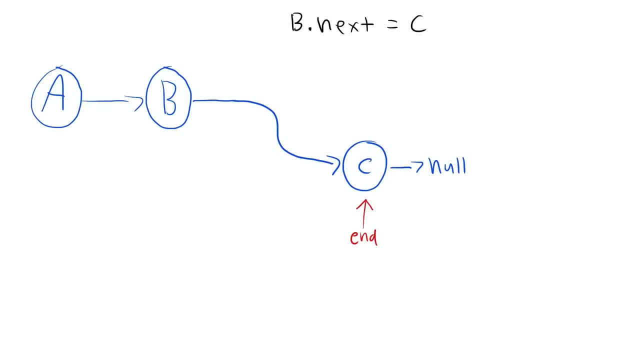 click the link below and you click it and then it installs a virus onto your browser. If a node's next pointer points to null, it's the end of the list. You can add a new node to the list in constant time by just setting that pointer to the new node, By doing additional. 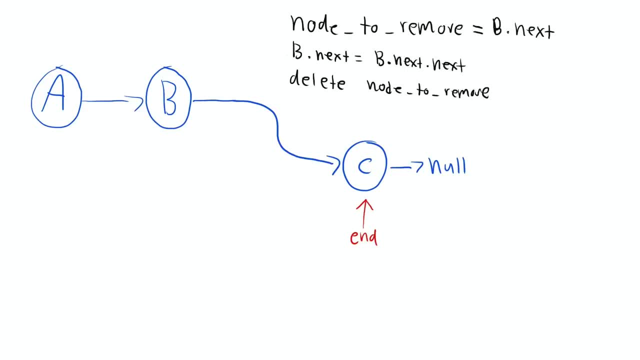 tomfuckery with pointers. we can also insert and delete nodes in constant time. Sometimes nodes also contain a pointer to the previous node, in a variation called the doubly linked list. But a major downside of linked lists is that you can't access elements in constant time via index. 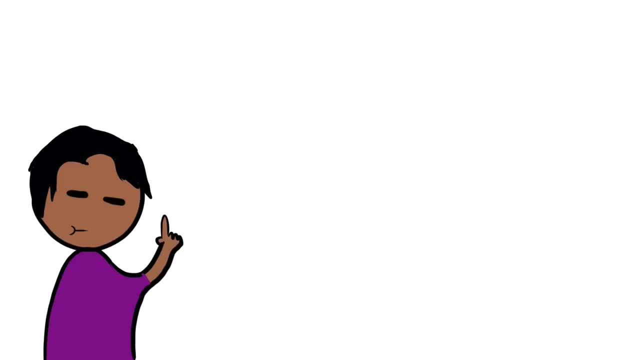 like an array. In practice, most programming languages have dynamically sized arrays or lists, which work by creating arrays with a fixed size. If the array is full capacity and you try to add a new element, the programming language automatically creates a new array with double the capacity. copies the current elements over. 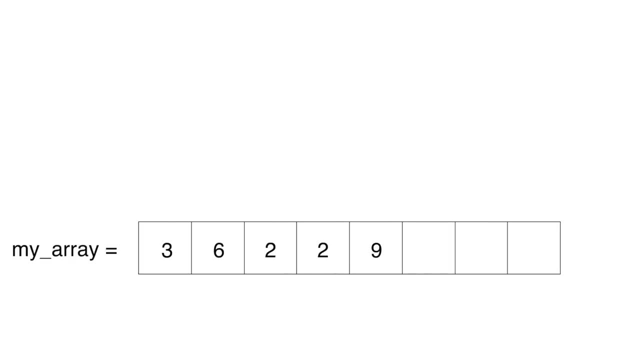 and sets your pointer to that new array. Since this happens so infrequently, we generally consider appending to a list to be a constant time operation. Linked lists aren't the only data structure that include nodes referring to other nodes. What if, instead of pointing to a next node, nodes pointed to a left and a right child node? This is: 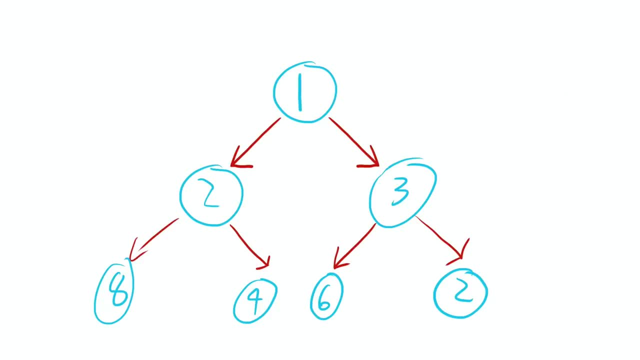 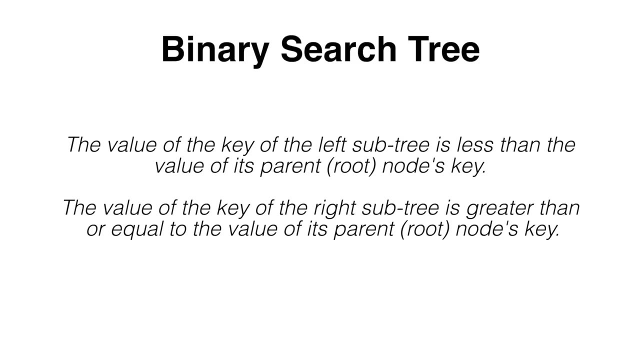 called a binary tree. These child nodes can also be called subtrees, since trees are recursive in nature. A node with no children is called a leaf node, while a node with 7 children is my f***ing father-in-law. A common type of tree is the binary search tree, which follows these rules. 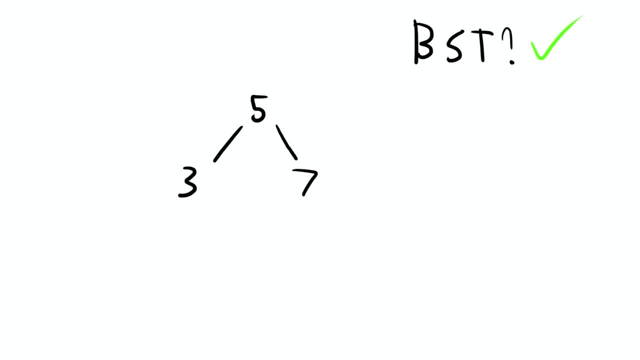 Basically, a node's left child must have a smaller value, while a node's right child must have a greater or equal value. Let's say you're looking for element x. You start at the root and if the number is smaller than the root you go to the left tree if it's larger. 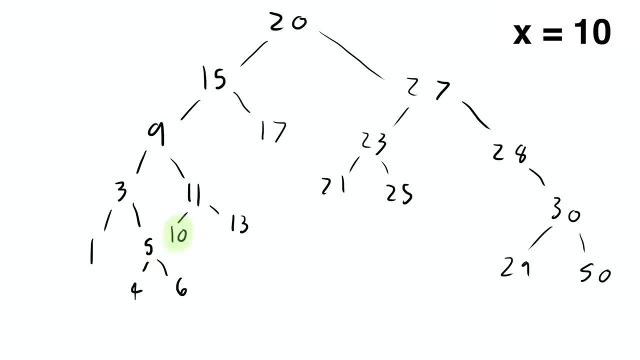 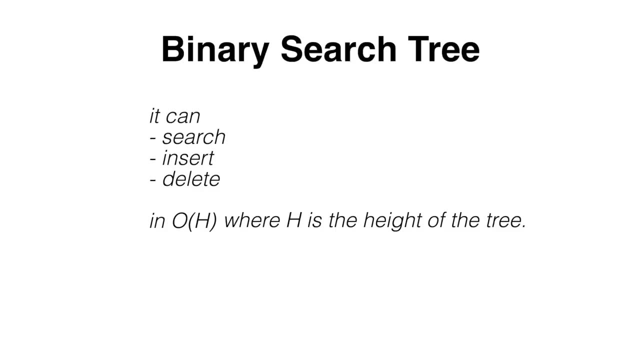 you go to the right and you keep repeating this until you arrive at your number. In the worst case you have to traverse the height of the tree. So the time complexity to search, insert and delete elements is O, where h is the height. This is efficient because, on average, 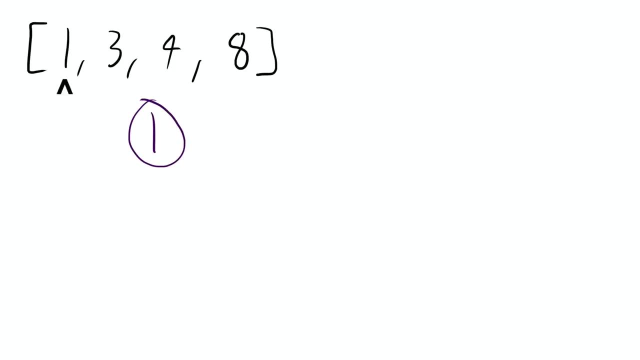 the height will be log n. But what if you inserted every element of a sorted array into an empty binary search tree? Well, that's a linked list, meaning the height would be n. But we can guarantee log n time complexities using a self-balancing binary search tree, such as red-black trees. 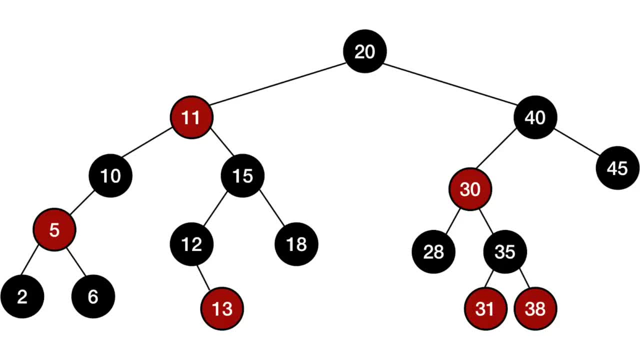 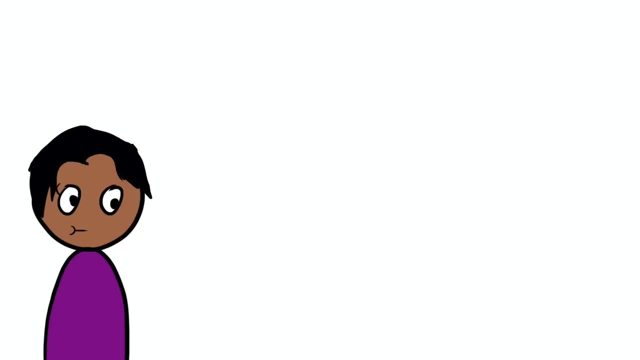 which maintain additional properties to guarantee that the height of the tree is O. Binary search trees are kind of considered to be a workhorse to researchers that can solve most problems with decent efficiency. but I found situations where binary search trees really shine are when you're asked a question about binary search trees. 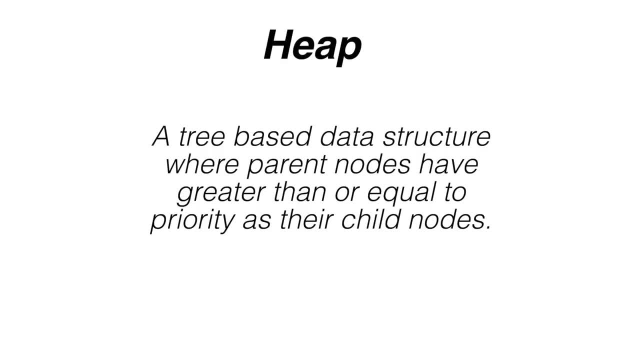 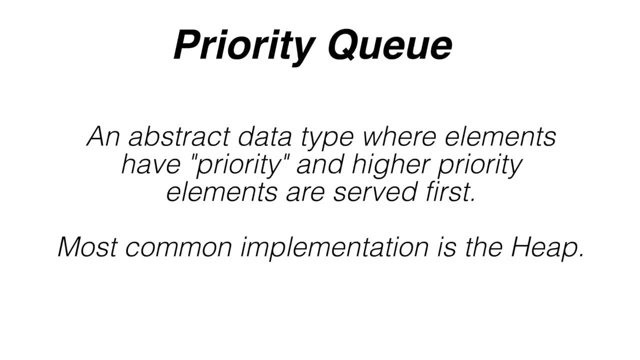 Another type of tree is a heap. The primary difference between this and the binary search tree is I actually use this one. It's also sometimes called a priority queue because at the root of it is always the highest priority element. A min heap will have the min element. 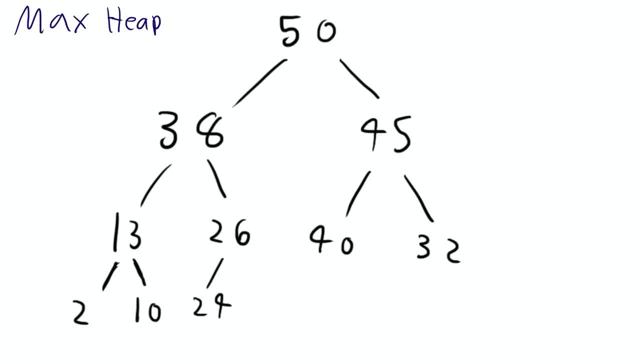 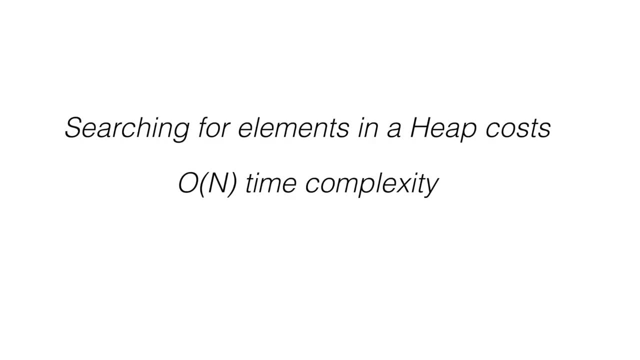 and a max heap will have the max element at the root. But don't get me wrong, the rest of the heap is unsorted. It is an absolute wasteland down there. Searching in the rest of the heap may as well be an unsorted array. We only care about what's at the 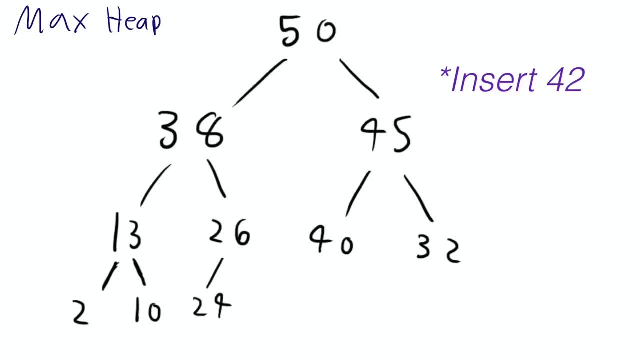 top. Just like capitalism, To insert a new element into a heap, first we find the next available spot to add a leaf node, Then we compare it with its parents and if it's a higher priority it swaps and bubbles its way up. We are doing at most log n comparisons. 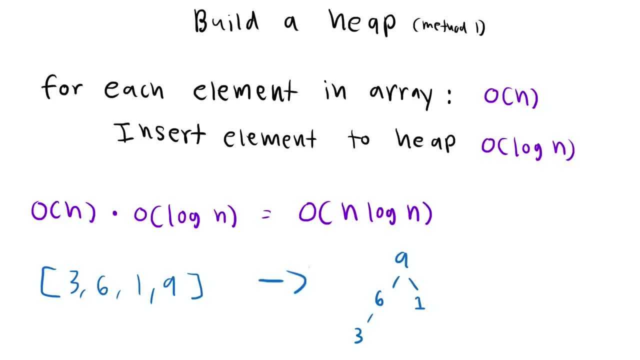 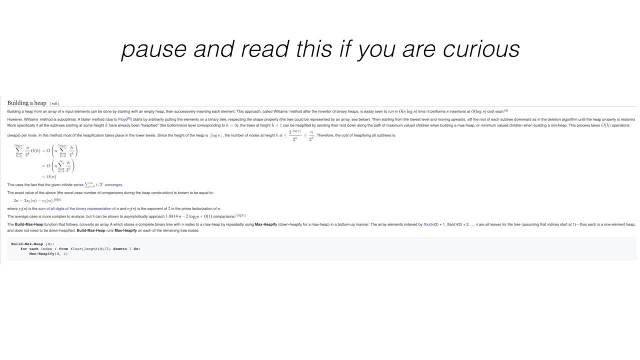 You can build a heap from a random collection by inserting n times, which costs O, but there's also a way to build a heap in O. I'd suggest reading this Wikipedia page because it's super interesting stuff If you're interested in learning more about binary search. 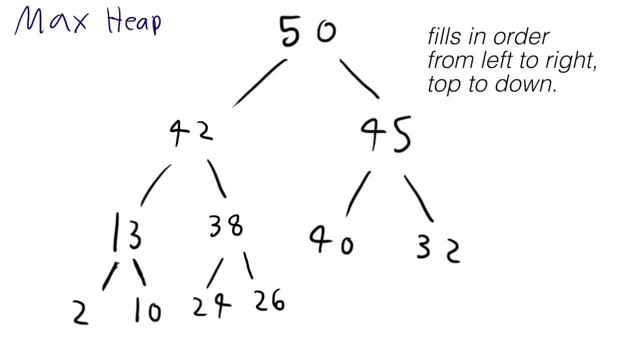 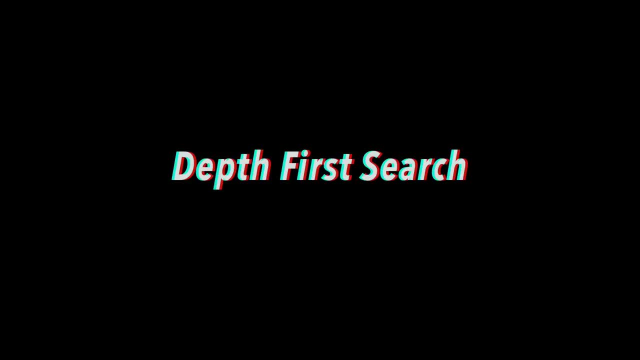 you can click on the link in the description. And lastly, since the heap is nearly complete, although we can visualize it as a tree, we could actually use these properties to represent it with an array. One way to traverse a tree is a depth first search, which is like going deep fully. 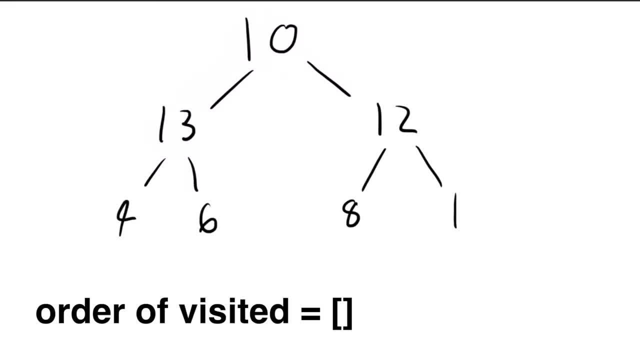 exploring one path and then moving on to the next. One way to visit this tree in a depth first order could be to start at 10,, go to 13,, go to 4,, then 6,, then 12,, then 8,, and then 1.. Whereas, 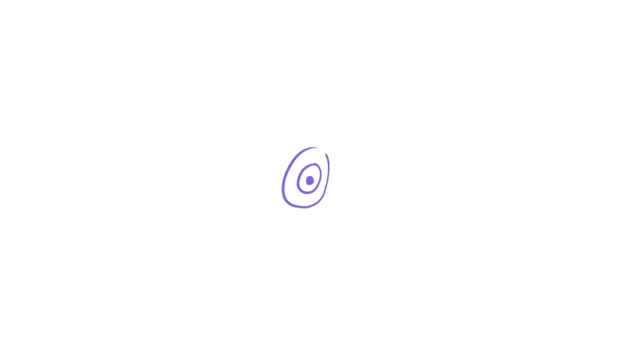 another option is a breadth first search, where we view it more level by level. A way to print this tree in a BFS manner could be 10, 13,, 12,, 4,, 6,, 8, 1.. When it comes to implementation, 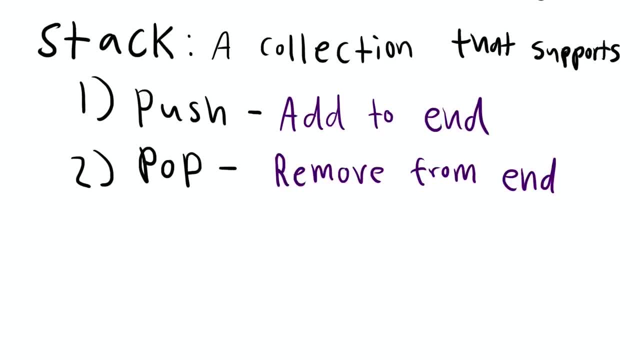 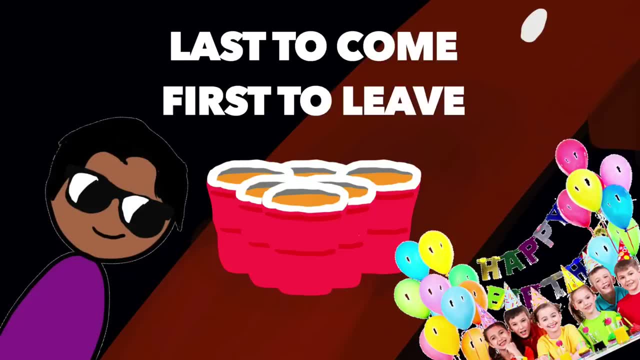 depth first search can use a stack. A stack is a list-based data structure where the only two operations are: add to the end and pop from the end. This makes a stack lefo last in, first out. DFS are often done using recursion which indirectly uses a stack, the recursive stack. 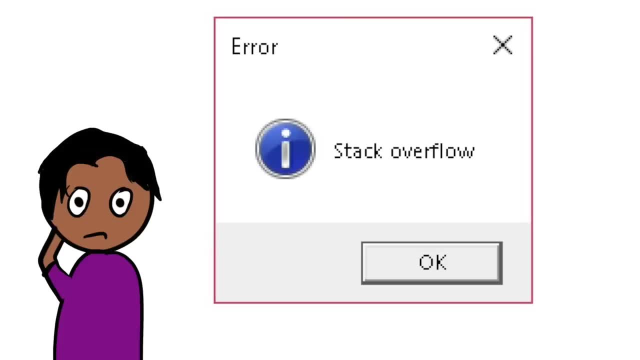 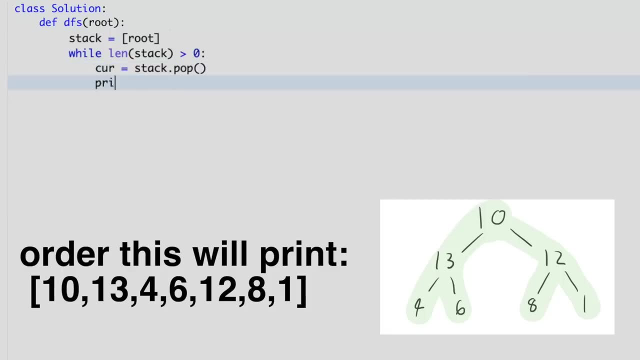 So if your recursion exceeds a certain amount of depth, then you get a stack overflow. Let's look at a way to print this tree in a DFS manner using a stack. So first initialize the stack and add the root. Then, while there are, 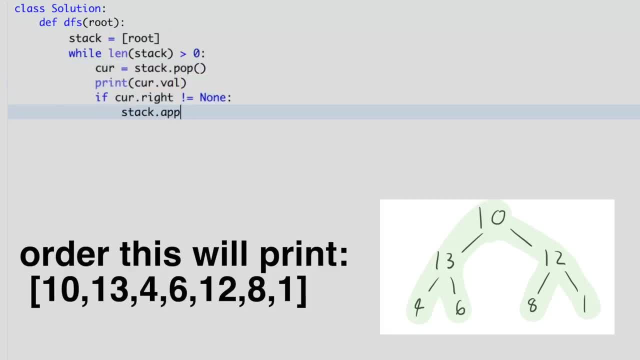 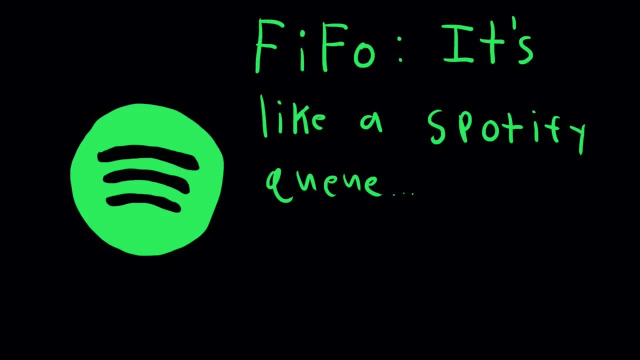 still elements in the stack, pop from the stack, print that element and then add its children to the stack. On the contrary, a breadth first search uses a queue. A queue is FIFO: first in, first out. So instead of popping from the end of the list, you pop from the beginning, Doing the same algorithm. 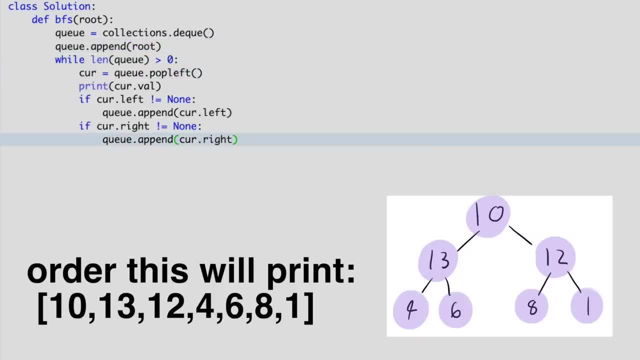 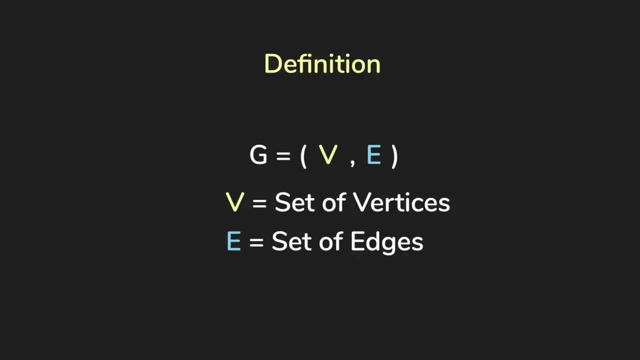 as before, but using a queue instead of a stack. the tree will now print in a BFS order. All trees are graphs, but not all trees are graphs. All trees are graphs, but not all trees are graphs. All graphs are trees. A graph is a collection of vertices which are like points and edges. 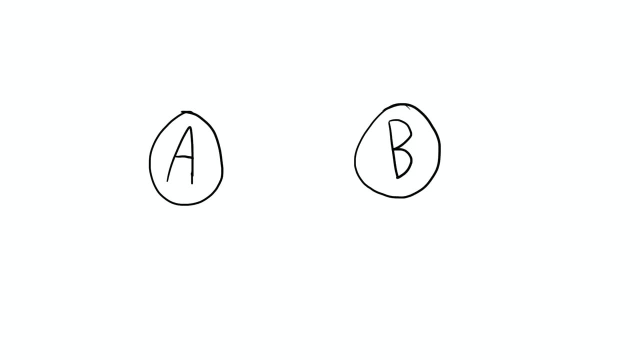 which are like connections from one vertex to another vertex. A graph can be directed, meaning edges can only go one way. so this edge means you can only go from A to B, or undirected meaning you can also go from B to A. Two common ways to model edges are adjacency lists and 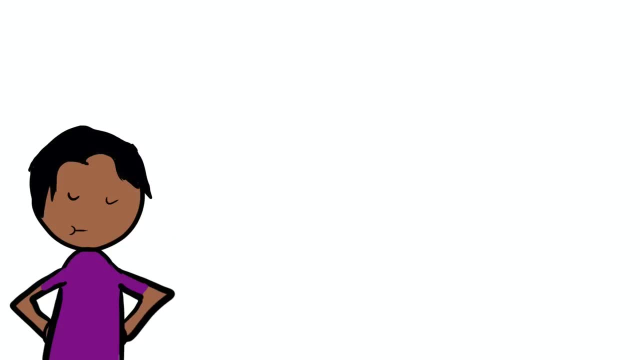 adjacency matrices. Graphs are my favorite part of data tracks and algorithms, so I'd like to show how cool they are with three example scenarios on where you can use them. So it recently dawned on me that I know Kanye West, and by that I mean I know Joma Tech, but Joma Tech knows Jarvis Johnson. 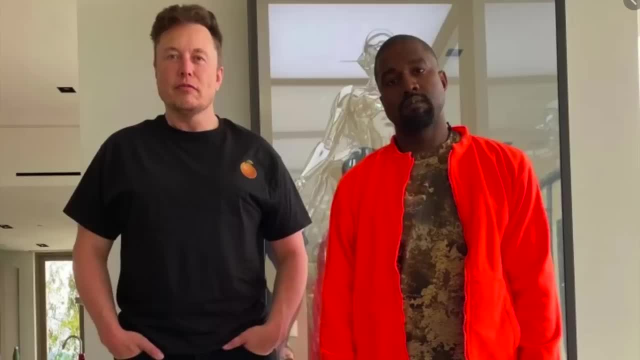 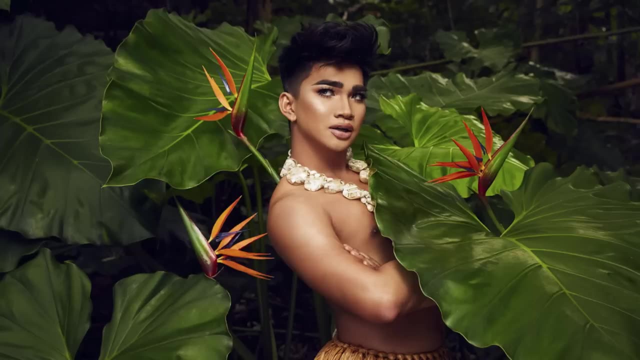 who knows MKBHD, who knows Elon Musk, who knows Kanye West? which is 5 degrees of separation between me and Kanye West. I wanted to find something shorter. Well turns out. I know Bretman Rock, who knows Rihanna? who knows Kanye? 3 degrees of separation, Which also 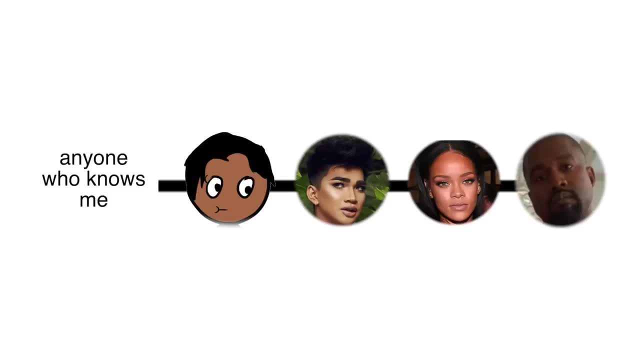 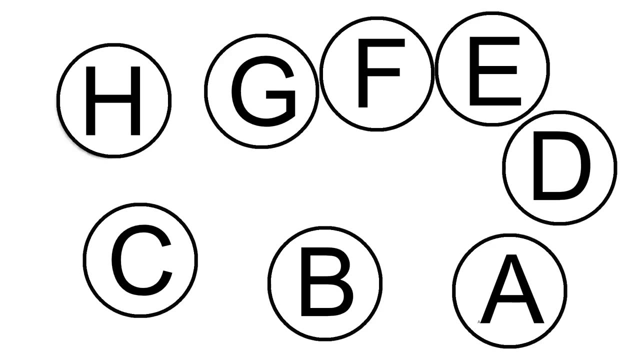 means that anyone who knows me is at most 4 degrees of separation away from Kanye. If we wanted to make a program that computes the smallest degrees of separation between two people, a graph would be the perfect choice. You model people as vertices and you model relationships. 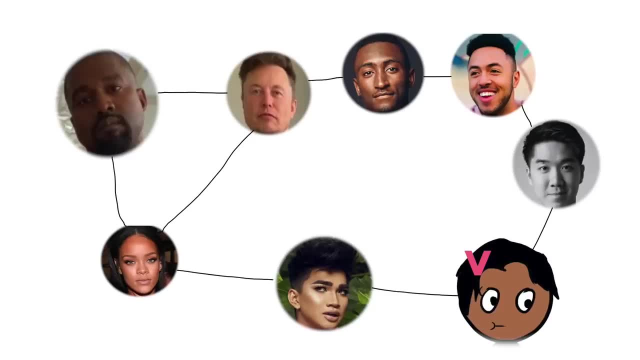 as edges. The shortest path between the source node me and the target node, Kanye can be found with a breadth-first search. Since we're moving out level by level, we can guarantee that the first time reaching the Kanye node will also be the shortest path. The problem with implementing: 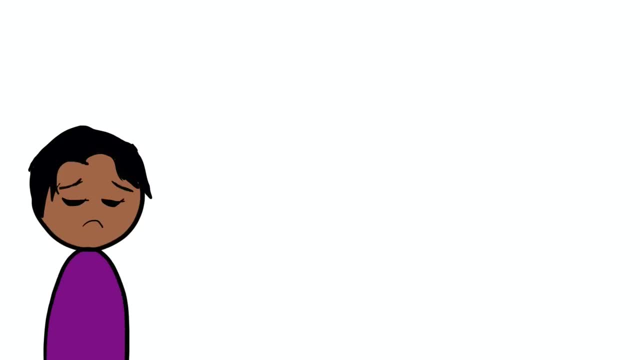 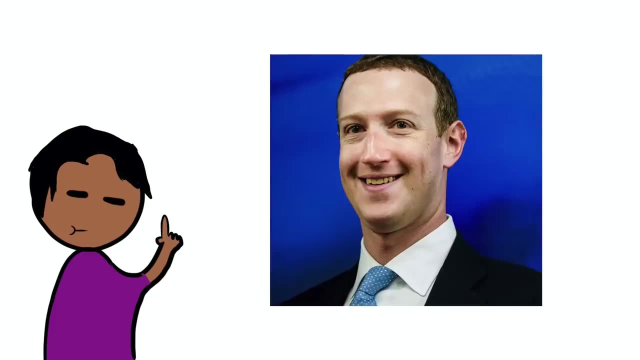 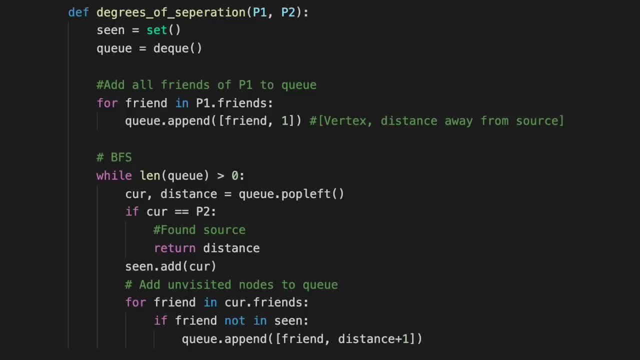 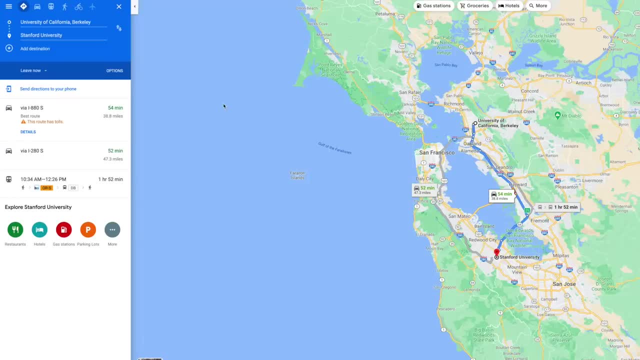 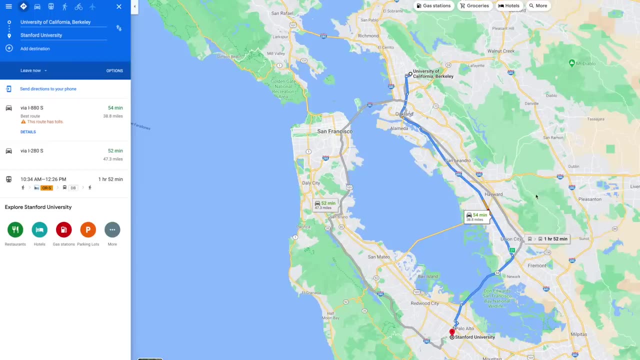 Imagine a map system like Google Maps that wants to find the shortest path between two locations. This is different than the last example because, although they both deal with shortest paths, the degrees of separation did not have weighted edges where a map system does, For example. 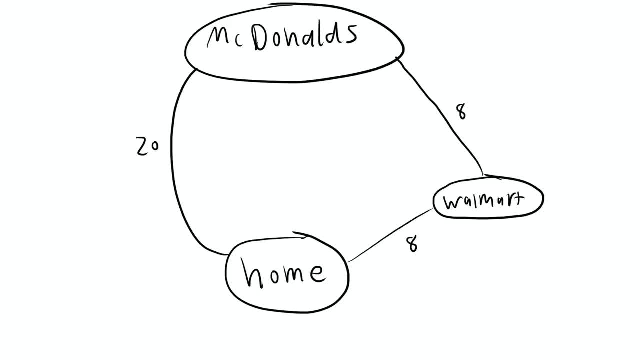 if we're computing the shortest path between two vertices and there's a direct edge between them weighing twenty, versus a path of two edges weighing eight each, a breadth-first search would give us the shortest path in terms of vertices away, but not the smallest weight. 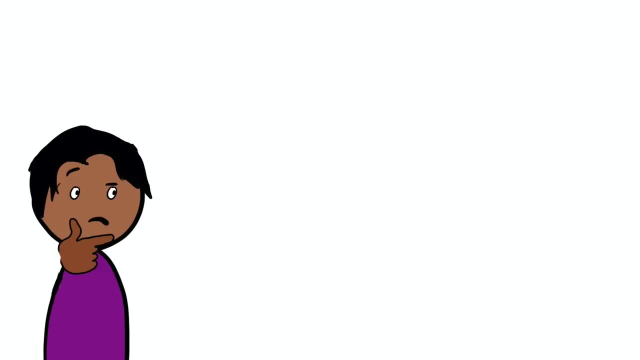 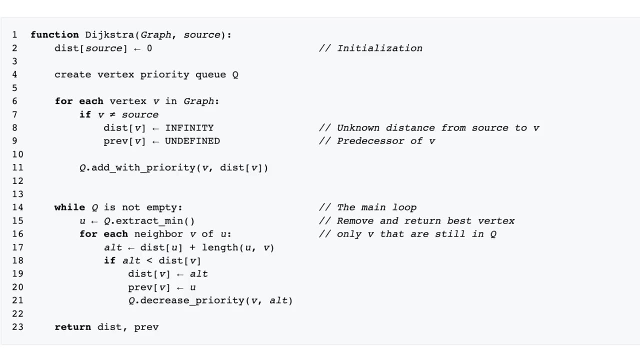 One algorithm that computes the shortest path in a graph with positive weighted edges is Dijkstra's algorithm, using the heap data structure. In the original version of this video, I explained Dijkstra's and my video shot up six minutes, so instead just research it for yourself if you're interested. 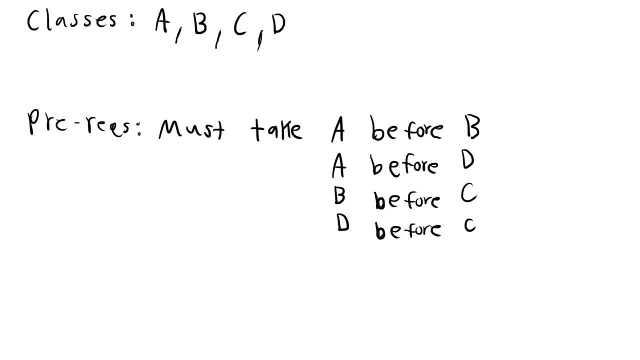 But graphs aren't just good for pathfinding. Imagine a course schedule in school with classes and prerequisites for each class, and say you wanted to find the order in which you can take all your classes while still fulfilling your prerequisites. Well, model the class. 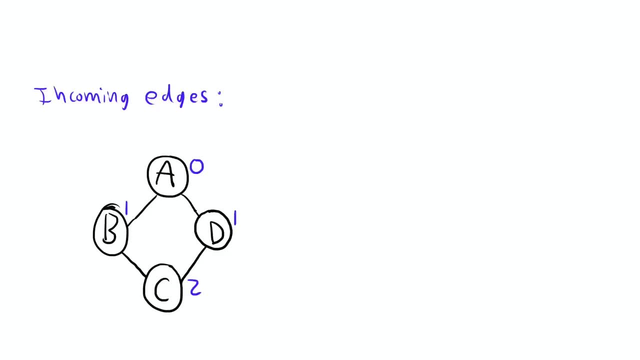 as vertices and prerequisites as edges Count how many incoming edge each vertex has. Add vertices with zero incoming edges to a queue. Then pop and print the element from the queue and decrement the incoming edges of all its children. If a child now has zero incoming edges, add it to the queue. 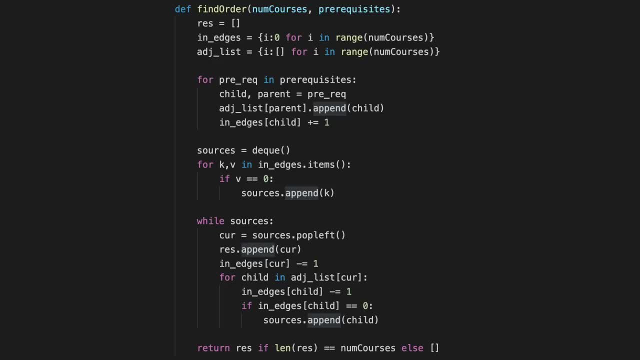 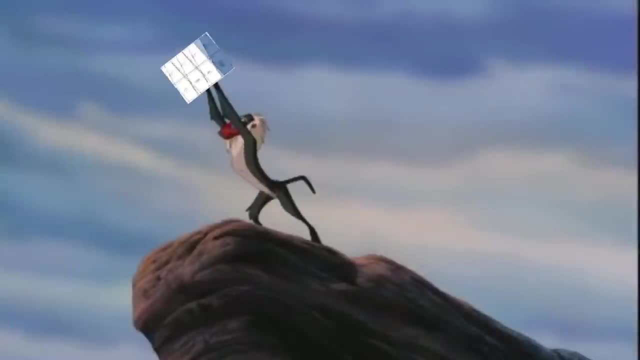 and repeat while there are still elements in the queue. This algorithm is known as the topological sort. Hash maps are sort of the holy grail of data structures With basically constant time retrieval of data. the saying goes that if you don't know what you're doing, just try throwing. 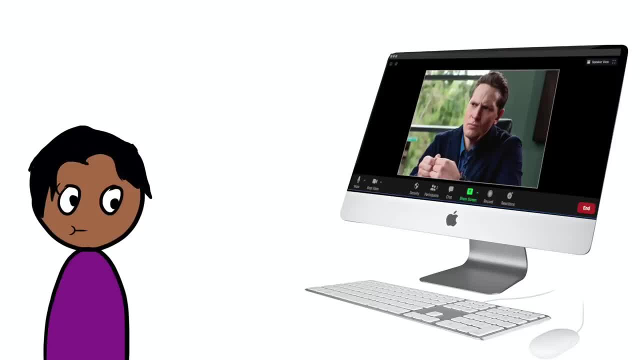 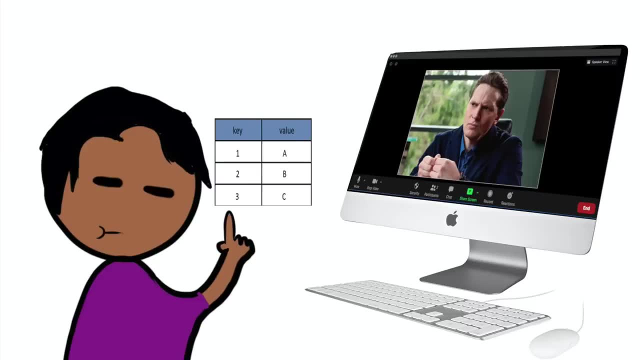 hash maps at the question As an example. one time I was in a coding interview and froze, so I just told the interviewer: hmm, I think the solution is to use a hash map. Unfortunately, the question was: what are your biggest weaknesses? So the better answer was: hang up the phone to show. 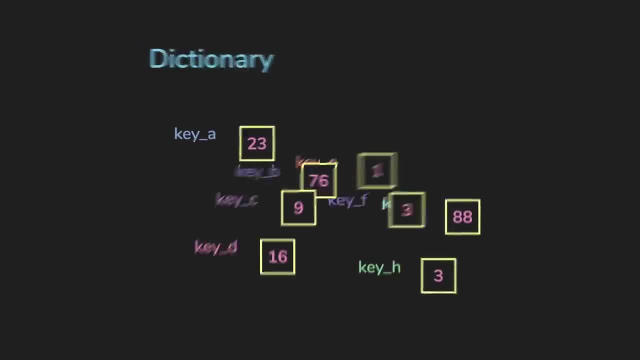 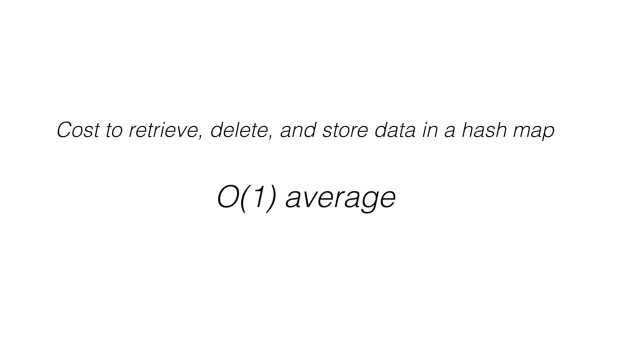 that I have none. A hash map is a data structure built on top of an array, optimized to store key value pairs. What makes it so powerful is you can retrieve, delete and store data in on average, constant time. Here we have a map where keys are strings representing people's names and values are. 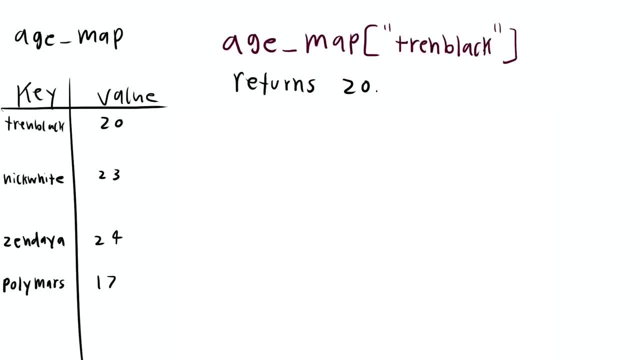 their corresponding agents. We can directly access TrendBlack's age like this. It's almost as if strings can be used as indices. But how is that even possible? Because of this little thing called a hash function. A hash function will take a key and return a hash code. If we take that number and modulus the length of 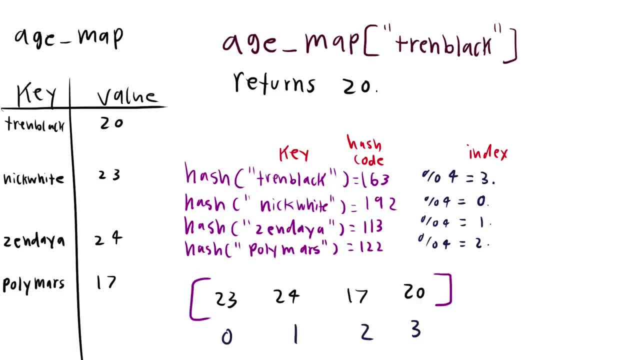 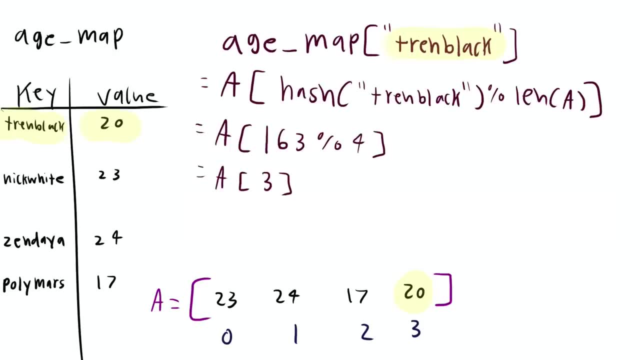 its underlying array. we can use that as an index to store its value. But the hash function has to compute the same hash code if given the same key. So hash of TrendBlack should always return the same hash code or else we lose the index. But what if hash of TrendBlack and hash of Ziz both end with 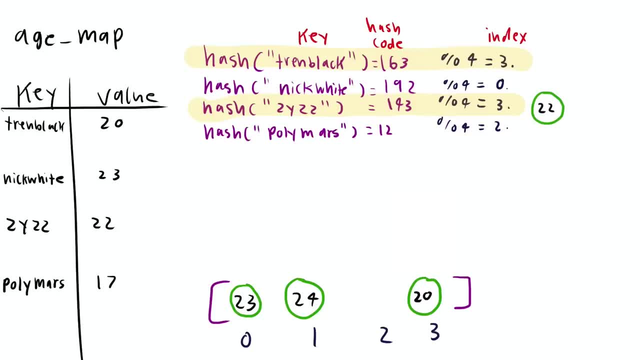 index. Well, this is called collision. One way to deal with this is to store our value in a link list. So when we go to store Ziz and see that index 3 already has a value, we have that value. point to the new value. This is why a hash map is not strictly O, because if you write some god, 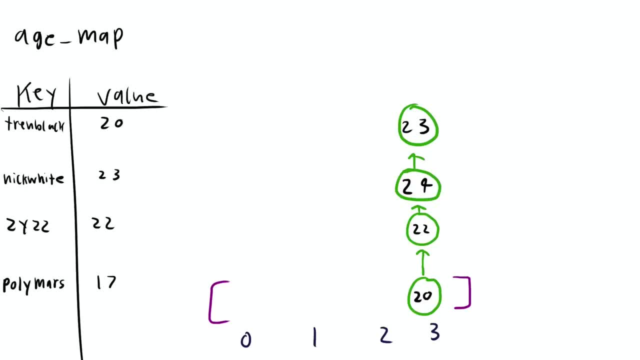 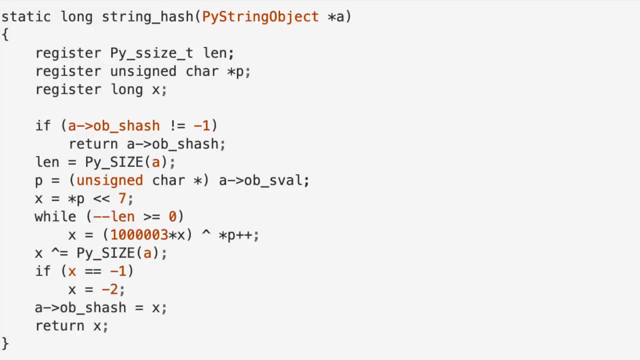 awful hash function, then it won't be balanced and we will have to do a lot of link list traversing Good hash functions. evenly spread out hash codes In practice. modern languages use very good hash functions so you don't have to write your own. An example of a hash map is the dictionary in Python. 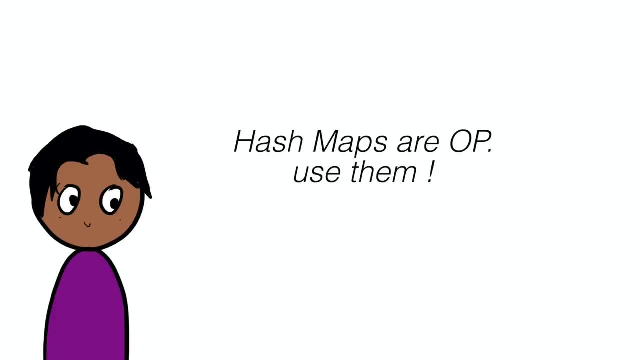 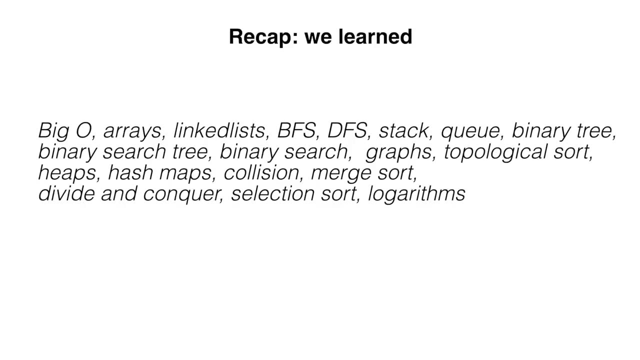 and the dictionary in JavaScript. And remember: constant lookup of data is very overpowered, so try to use it when you can, And that's pretty much all you need to know for data structures and algorithms. A 6 month college course taught in 13 minutes. Now, of course, you didn't learn anything. 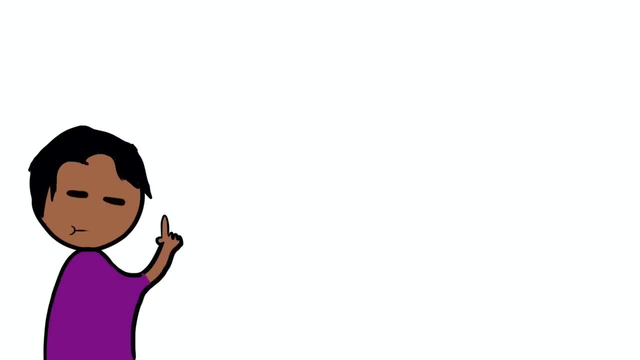 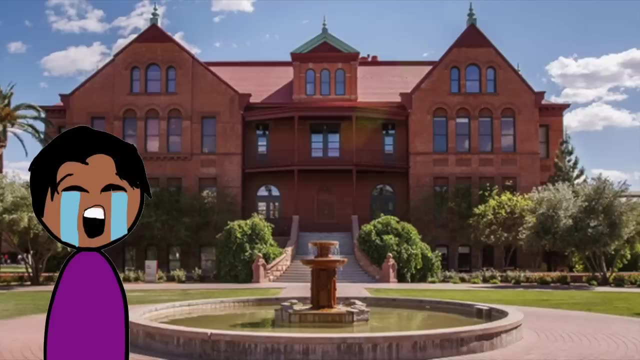 in great detail. but trust me, it is a lot easier to learn something in great detail if you already learned the big picture first. This is why college sucks at teaching. It dives very deep into one topic and then moves on to the next. It's like a depth first search. I believe the better way of 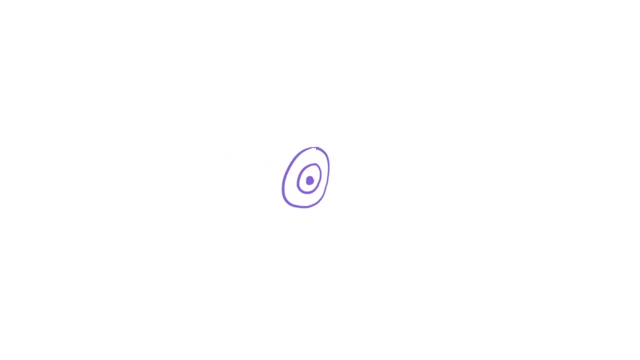 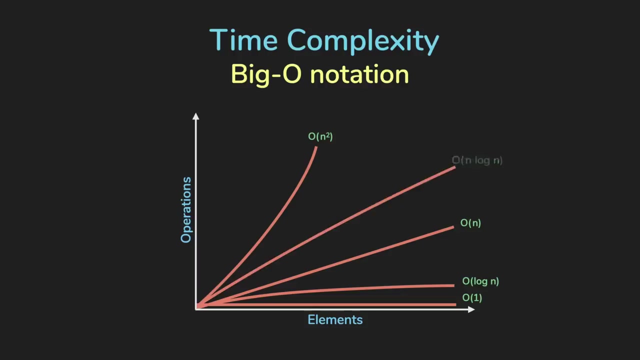 learning is to get a general understanding and then build on it Like a breath first search. So if you want to keep going, what are my recommendations to build on your knowledge? Well, the first one is JomaClass. You know those really nice animations in this video. 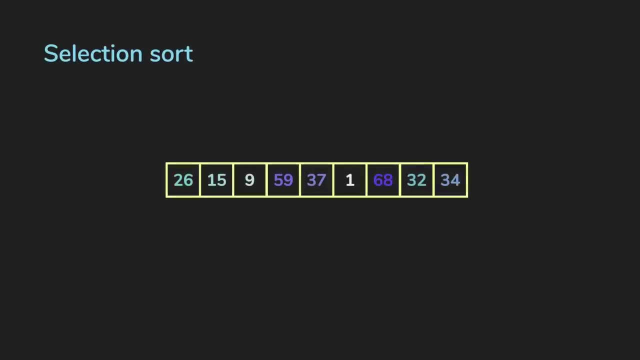 like this one. Yeah, I got them from JomaClass. If you don't care about getting extremely theoretical and just want simple, to the point, everything you need to know and nothing you don't type lessons, then JomaClass makes this difficult topic very accessible. But I will admit that I 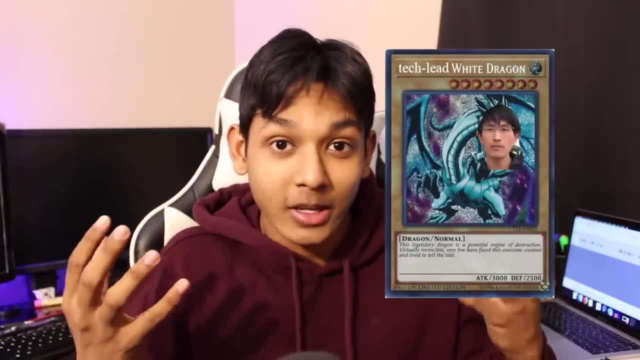 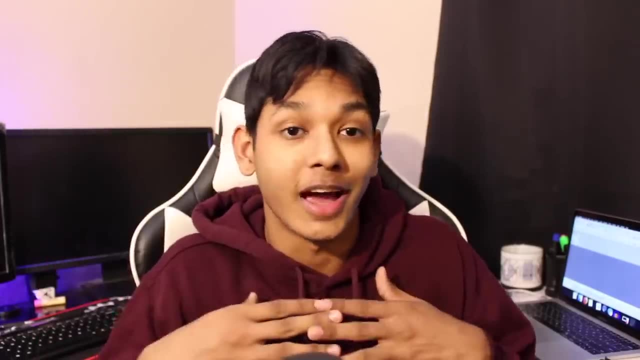 roasted the fuck out of Joma a while back because, if you don't know what you're talking about, he was pushing some actual snake oil. Well, unlike some people, he took my criticism very well and, to vindicate his name, he made something that is actually valuable and I will defend that.